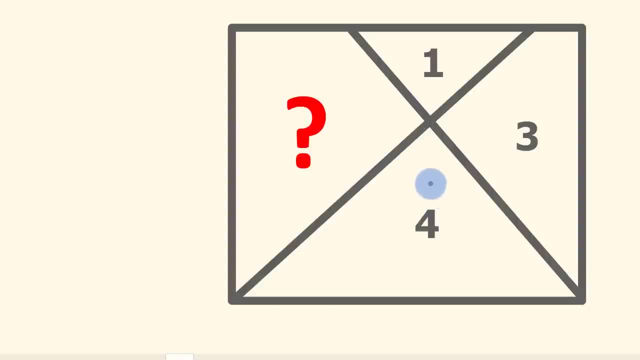 So, to start off, let's have a look at these two triangle parts here, the one with the area of four and the one with the area of one. It's apparent that these two triangles are similar to each other, That is, they have the same area of four and the one with the area of one. 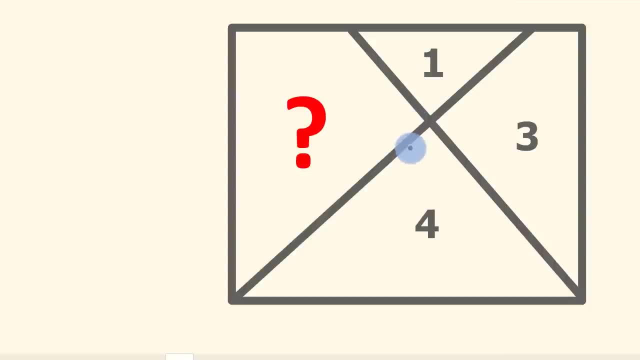 They are the same shape but they are different sizes. And we know this because we can work out the angles of these. First off, where we have these two lines intersect. here we have vertically opposite angles which are the same. We also have angles which are formed by a line running through parallel lines. 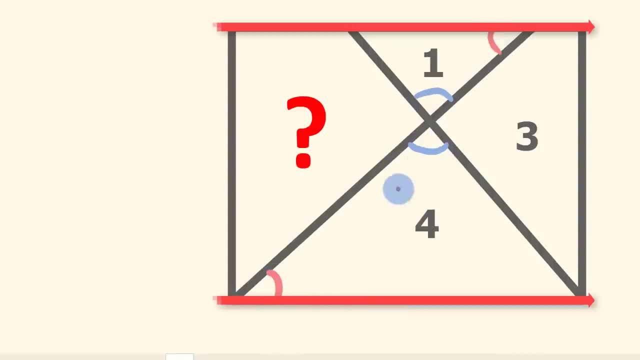 which form alternate interior angles, So these two angles are also the same. In addition, we also have this line which runs through these two parallel lines here of our triangles forming two interior angles that are also complementary to one another. So, as you can see, this angle matches up with this angle. 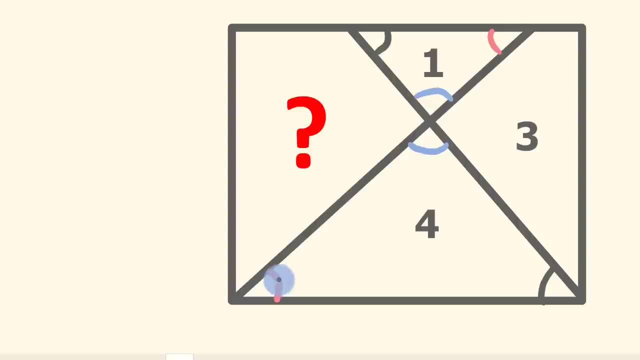 This angle matches up with this angle, This angle matches up with this angle, And what we're left with is two similar triangles. So now what we can do is we can compare the areas of these two triangles. These areas are in proportion to one another. They are in a four to one ratio. 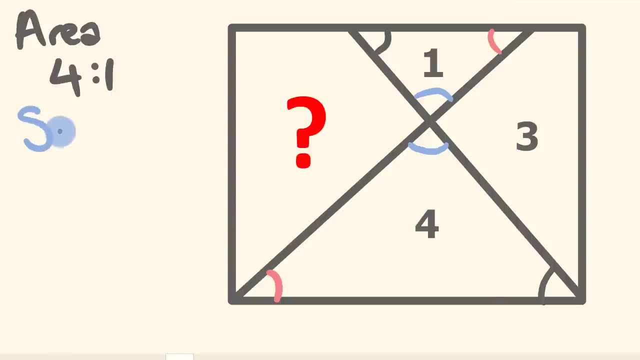 What this means is something pretty special. What it means is that the sides have a ratio of two is to one, because area is proportional. It is a side length squared. And I'll tell you what I mean by that. If we were to have a triangle, and that triangle was to have a side length of six, 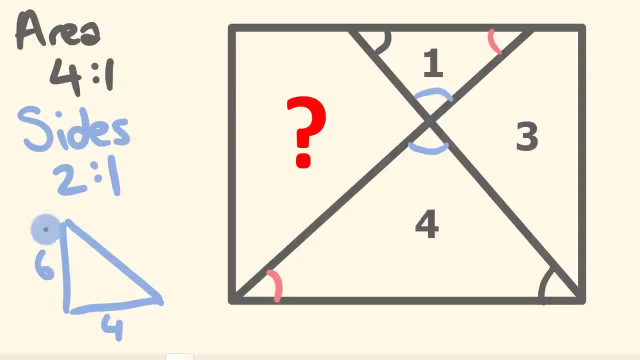 and this one was to have a side length of four. we could easily work out the area by going length by width, divided by two, Six times four, which is 24, divided by two, which is equal to 12.. Now, if I was to halve our side lengths, we'd have three and two. 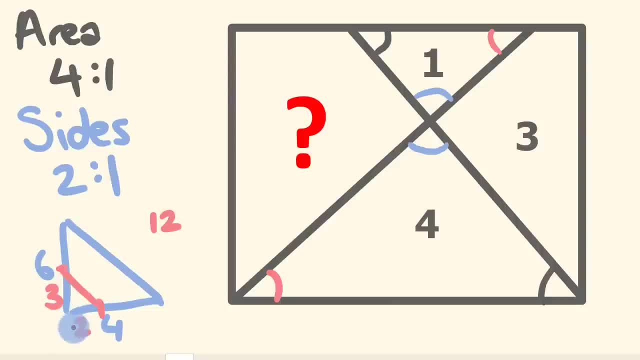 We could work out the area of our little triangle here. Three times two is six. divided by two is equal to three. You can see that our areas have a four to one ratio, But our side lengths have a two to one ratio. So we can use this now to solve our problem. 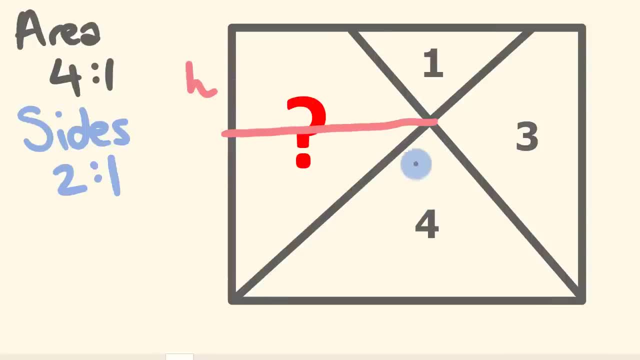 If we call the height of this triangle here h, it makes the height of the bigger triangle two h, And so I can actually break this up now into two rectangles. We have a rectangle here, and we also have a smaller rectangle up the top here.